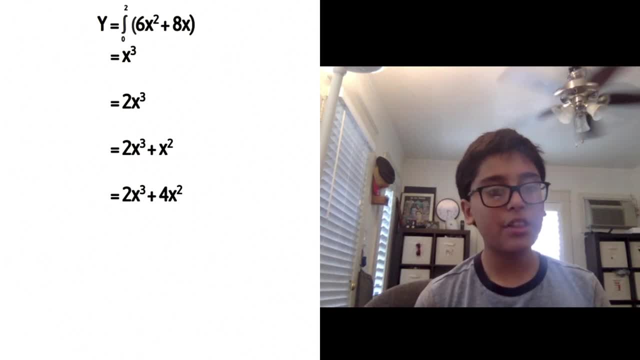 It's 4.. What's 2 to the 3rd power To the 3rd power is 8. Times 2. 16. What's 2 to the 2nd power To the 2nd is 4.. 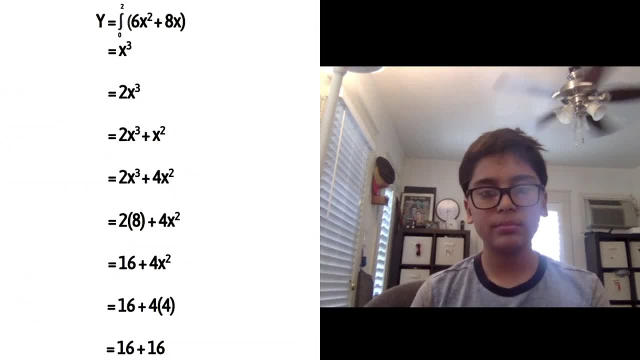 Times 4? 16.. Slok, you just learned chemistry: Calculus in 60 seconds. 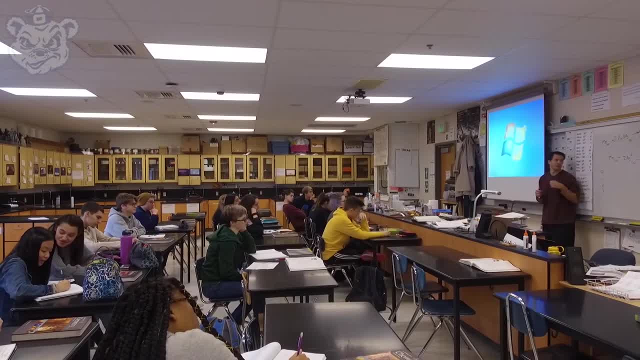 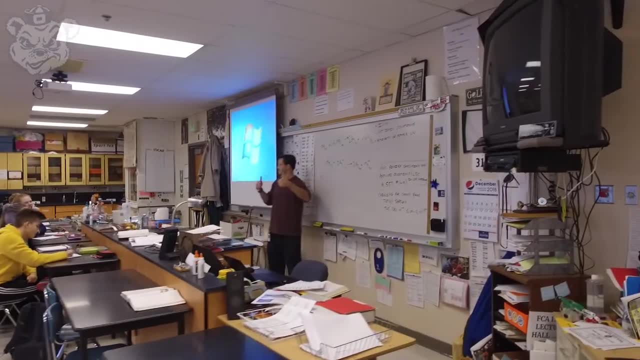 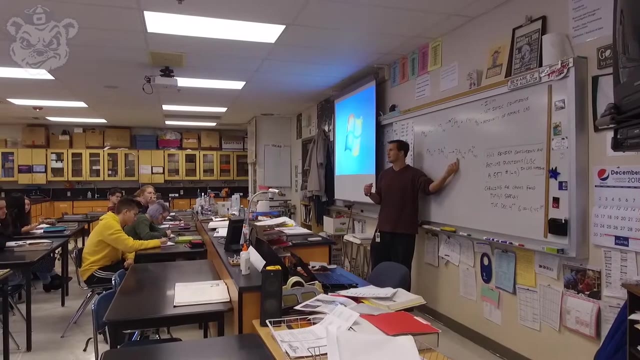 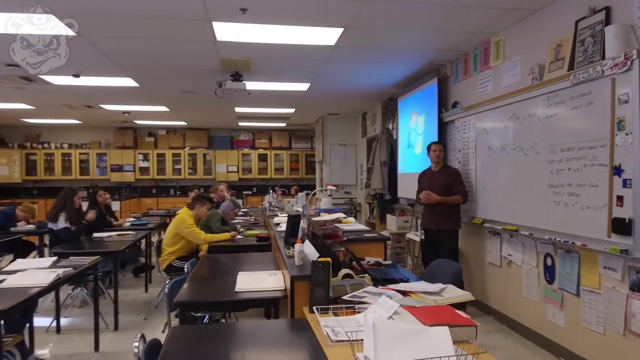 And this terminology is trickier, which is why we want to practice with it. So those of you who said that magnesium is being oxidized right to that two plus charge, that is correct. Okay. So magnesium being oxidized and the silver in this case, is being reduced, or reduced to its elemental form. That's what the terminology came for. Okay, Reduction in charge to the elemental form. So anytime we have something being oxidized in the direction, we're also going to have to do it. 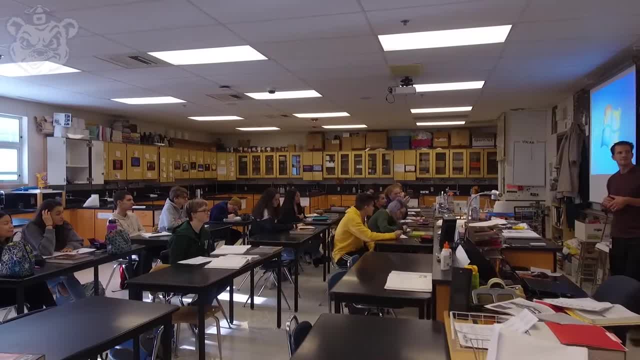 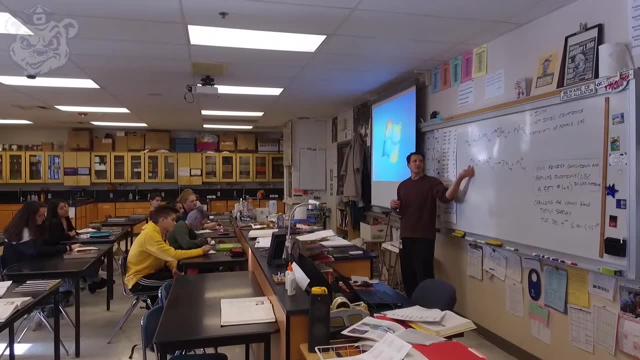 So I just don't understand why you're rewriting it. Like what's the point of talking about that? Well, when you start looking at the actual energy that's associated with our magnesium as a metal going to a magnesium ion, because we're actually going to get like an electrical 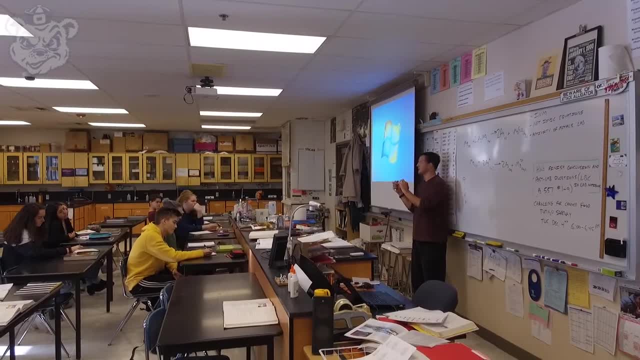 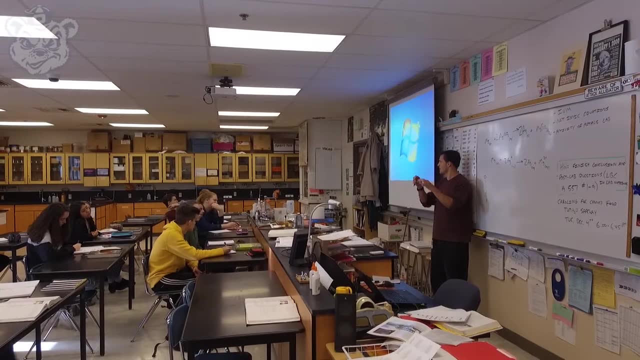 charge that comes from that, from those two electrons that are being donated to our silver right here. So we're actually able to like, stick electrodes in a line to see how much electrical potential deficit is in that, Yeah, and so we want to be able to separate it out. 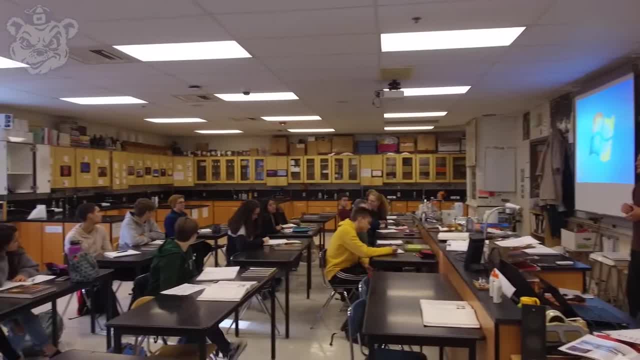 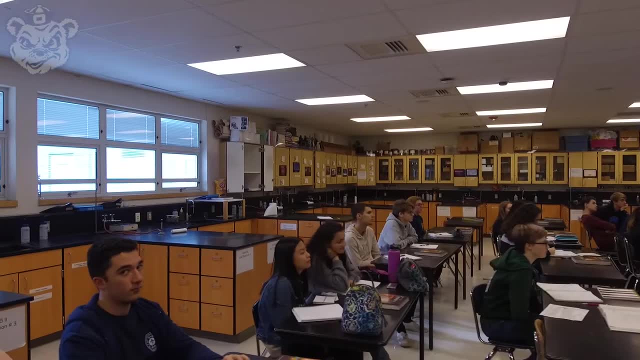 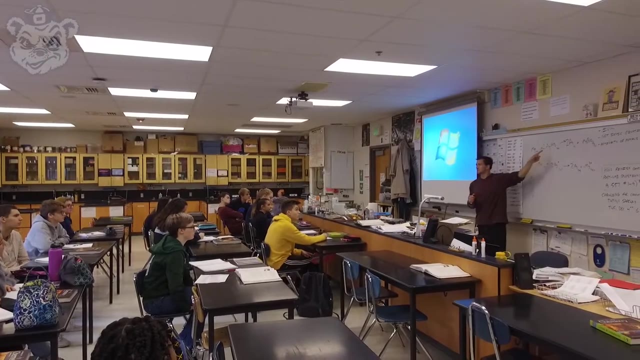 Okay, All right. Well, this might be exactly what you just asked. I'm not so sure. But I still don't get like why the energy is going to the spectator, Why we call it like a spectator ion, Because it just stays aqueous, So all we see happening. 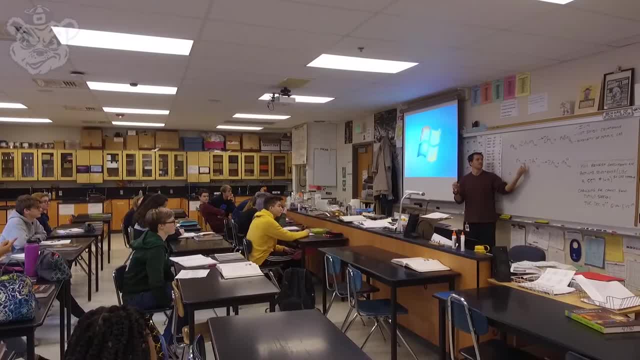 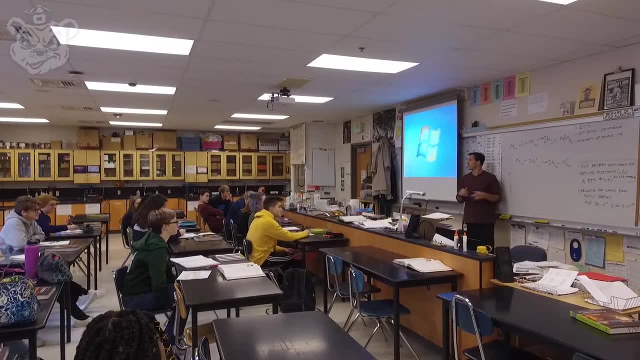 is the passing of electrons from magnesium to the silver. So if it doesn't change the state, it's a spectator Right, Or if it doesn't, actually It doesn't become part of the. So in this case we have, you know, the precipitate.